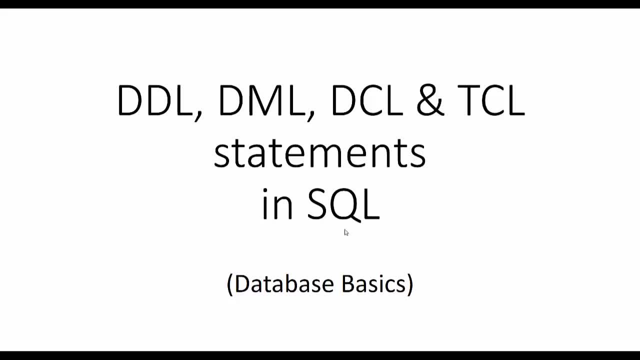 give you a brief description about these. So, in SQL language, irrespective of the database tool like SQL Server, Oracle or MySQL, and if you talk in terms of the SQL standard- that- the ANSI standard, every SQL language has, you know some classified set of statements, right, And these are: 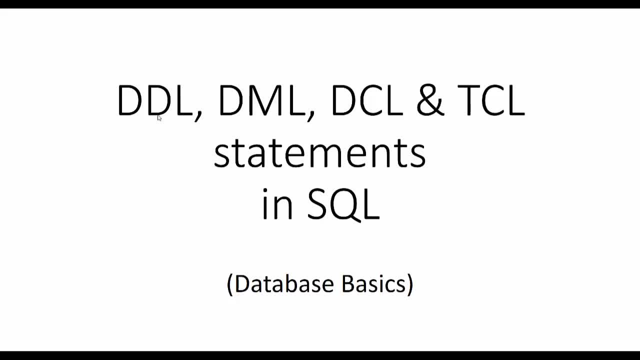 classified into different, different type of languages. right Like, like the DDL, that is the data definition language. Second one is the data manipulation language. Third one is the data control language And fourth one is the transaction control language. Okay, Okay, So first one is the. 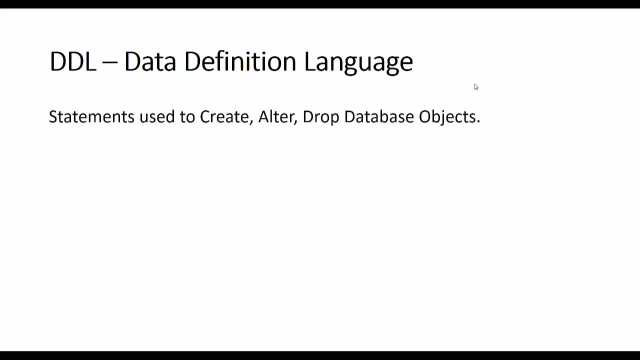 DDL, right, So DDL is data definition language. So by data definition language it makes clear that you know with this DDL you define your data means in SQL or any other SQL product like SQL Server, Oracle or MySQL. the data is stored in form of tables. okay, a relational table, So a DDL statement. 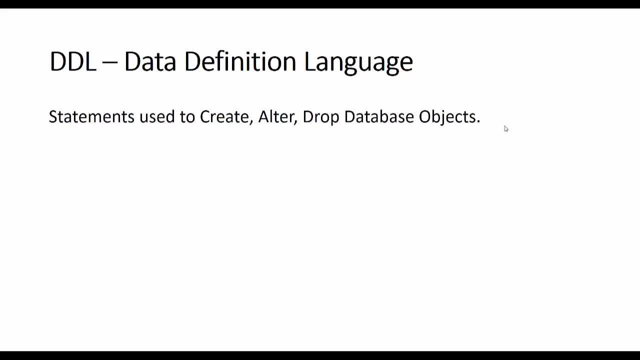 you can create, alter, drop the database objects. With the create statement, you can define new objects. Objects means tables, views, stored procedures and functions- right. With the alter statement, you can modify the definition of an existing object Like you can modify a table you. 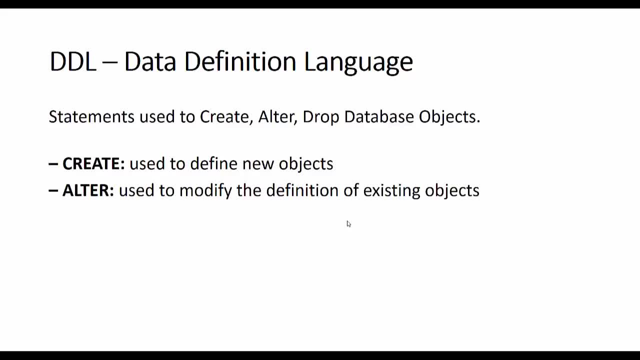 can add a new column in a table. You can modify the data type of an existing column right Or you can remove the column. also, with the alter statement, You can update the stored procedure. you can modify the stored procedure by using the alter statement. You can also modify the view definition. 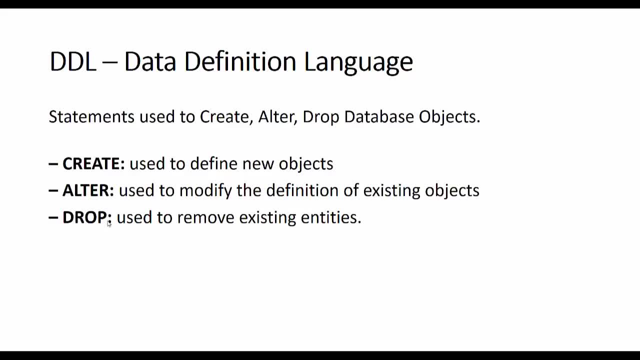 with the alter statement. The third is the drop statement. With the drop statement you can remove existing objects like: drop the tables. you can drop the views, you can drop stored procedures and functions. truncate table. truncate table is used to remove all rows from a table without logging the individual. 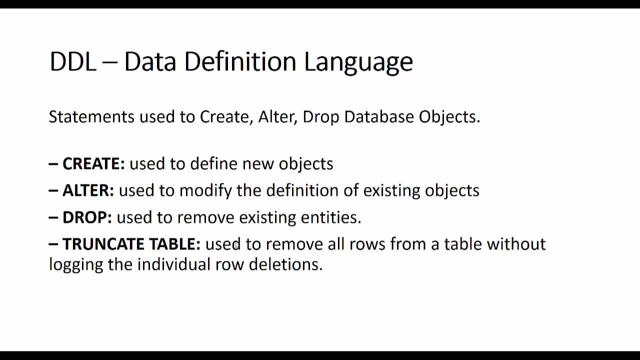 row definitions and this truncate table comes under. so this truncate table looks like a dml but it comes under ddl because it resets some properties of a table. so it is kind of a ddl because it redefines the definition of a table. for example, if you have an identity column in a table, 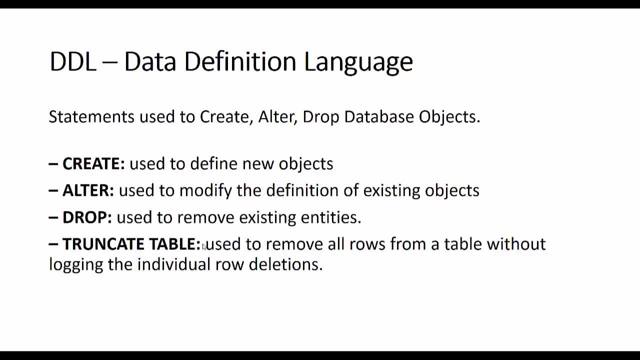 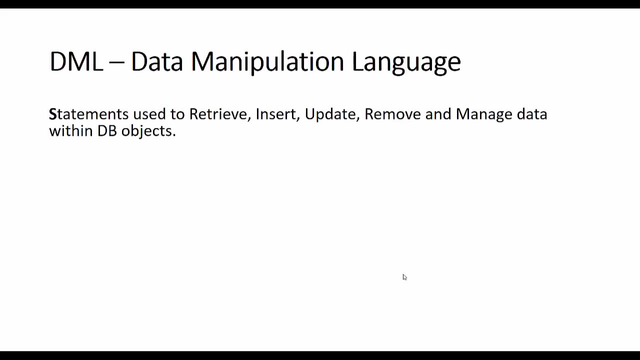 and if you are truncating the table which is having, which is having data, so it will remove all the rows and it will also reset the identity seed to the value that it was defined earlier, right when the table was created. so truncate table also comes under ddl. okay, now the second. 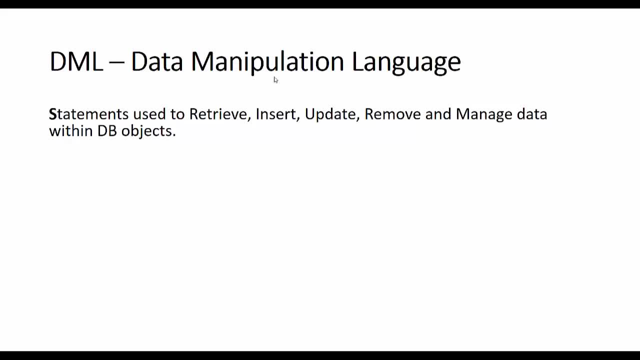 thing is dml, that is, data manipulation language. so with the term manipulation, it is clear that these languages are used to modify the data right, like the state of state of statement, used to retrieve, insert, update, remove and manage data within the database objects like the select statement. so with the select statement, a lot of people have, you know, some confusion. 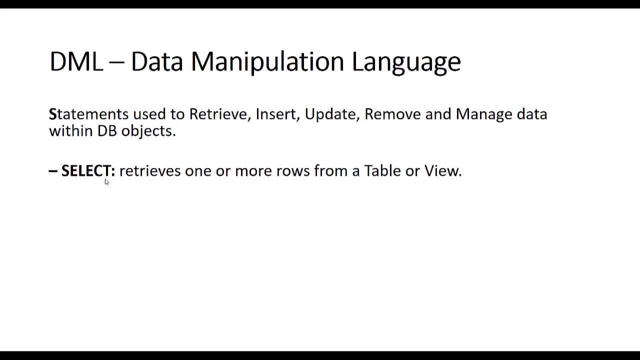 regarding this statement, that is select statement, a dml, because with select statement you just retrieve the data, you don't modify the data, you don't insert and you don't delete the data, right, but is a select a dml. so select is a dml because when you not only retrieve the data but you can 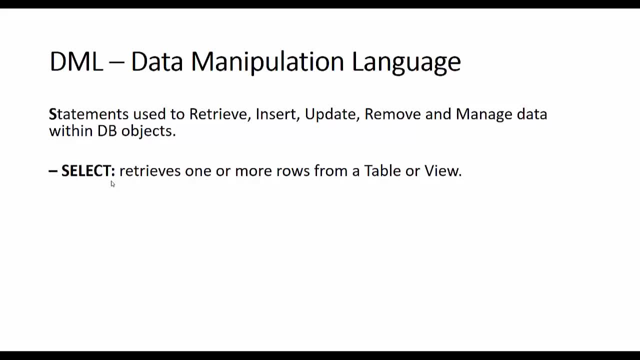 change the nature of the data, that you are retrieving it by using various functions that are provided in sql. by using aggregate functions? okay. by joining the tables and getting the meaningful data in some some other way? okay, so let's say you have a first name and last name. 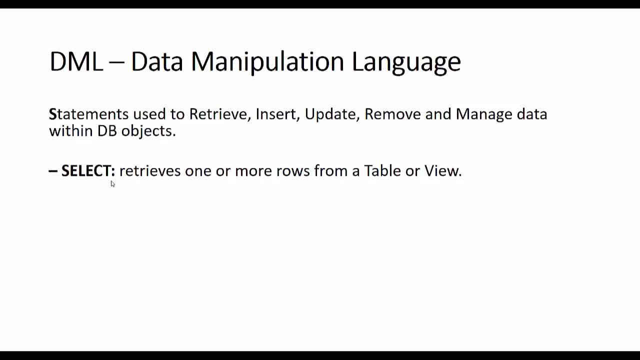 two columns and you can combine those two columns and get first name, last name as a combined name, right, like my name is manoj. manoj is present in one column, that is first name and pandey, my cast, is present in the second column. right, but you can combine both columns and can have a one column. 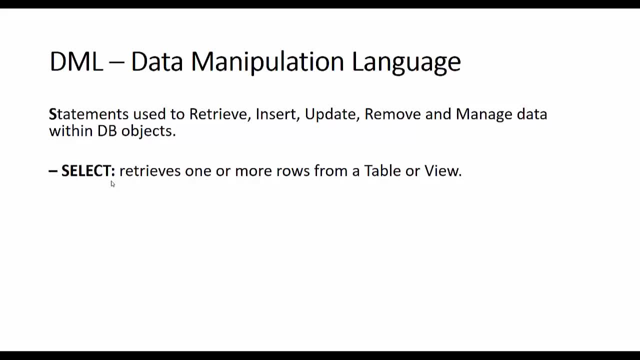 named that has a value as manoj pandey right. so here, with the select statement, you manipulated the data right that is stored in the. so the data that you are retrieving is different from the data that is stored in the table. second is the insert statement. insert statement: you used to insert one. 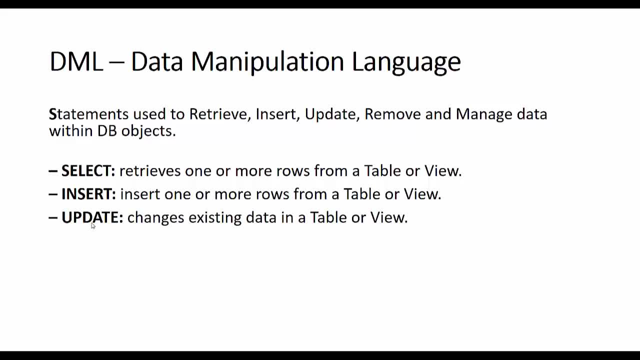 or more rows in a table. the update statement. with update statement, you can update the existing data that is present in the table. you can either update a row or you can either update multiple rows at once. you can also update multiple columns or you can update single column at once. okay, any combination of that. the deleted: 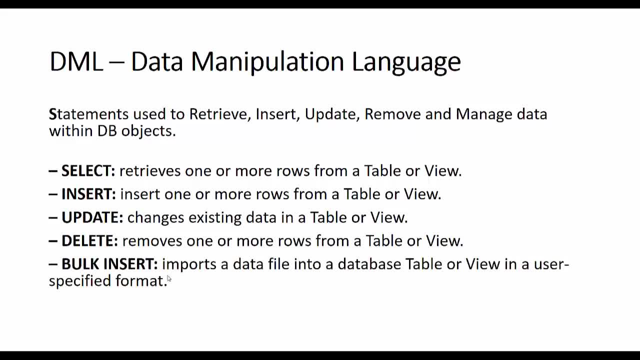 statement removes one or more rows from a particular table: bulk insert. so bulk insert is a utility that imports data from external files into your database table. okay, then the merge statement. so merge statement is a combination of insert, update and delete statement. so if you have to do these three operations at once in a in in a transaction, in a single transaction, then you: 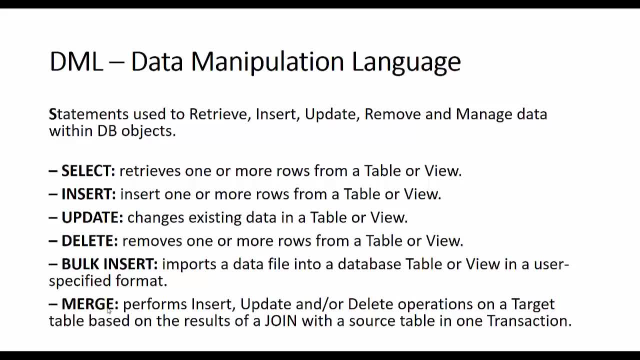 then you can have a merge statement. so this is based upon two tables. you have a source table and you have a target table. so if you have to keep both the tables in sync, so you can use the merge statement, right. we'll see in our coming videos about all these type of statements how. 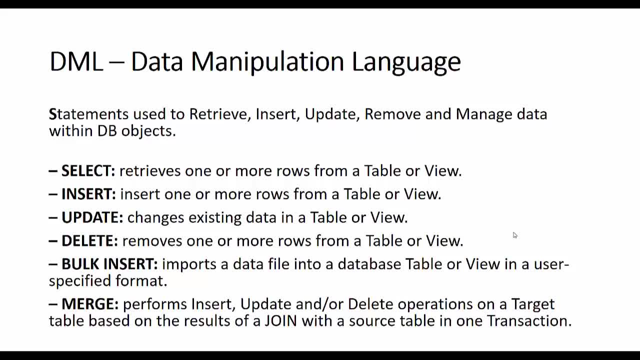 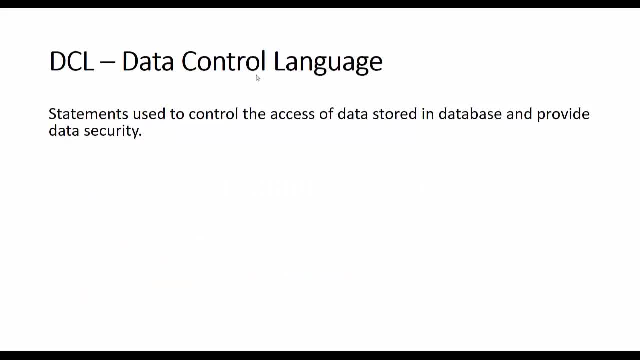 they work okay. so for now i'm just talking about at a very high level. uh, what exactly are these statements then? dcl, that is the data control language. as a database administrator, you can have some control on the data and you know this statement is used to control the access of data. 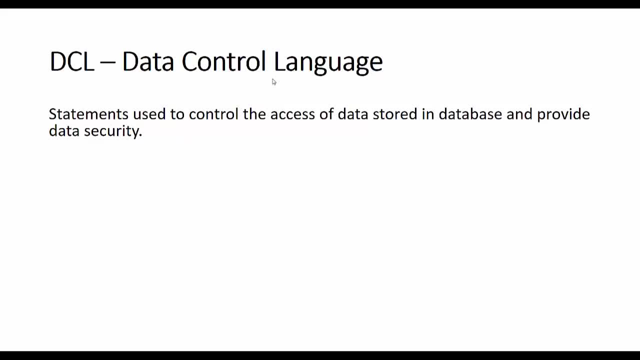 stored in database and provide data security right. so these ddls are under the control of dba, that is the database administrator. so first statement is the grant statement. so with the grant statement, a database administrator will be able to control the database administrator. so with the grant, 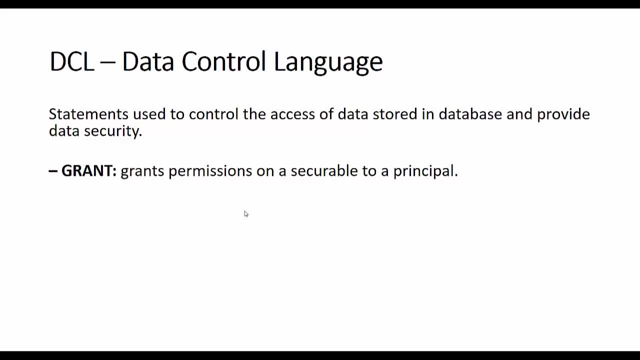 statement: a database administrator can grant permissions to other users to access the table. so let's say a dba can give grant permission just to select the data from a table so that user cannot update the table. right that user cannot insert a row, cannot update a row, cannot delete rows from. 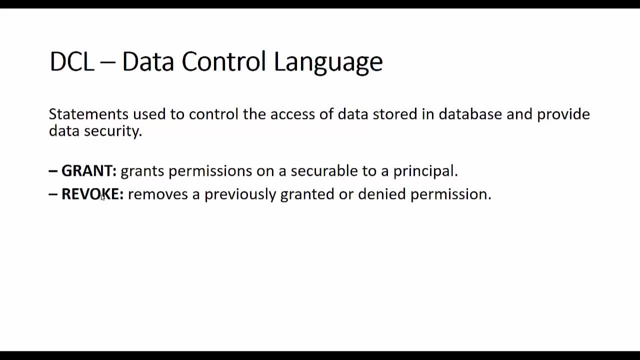 a table. he can only do a select from the table. revoke- revoke statement removes the previously granted or denied permission. so let's say the dba just wants to revoke that permission so that the user cannot be able to even select the data. so by using the revoke statement the user will not be able to do. 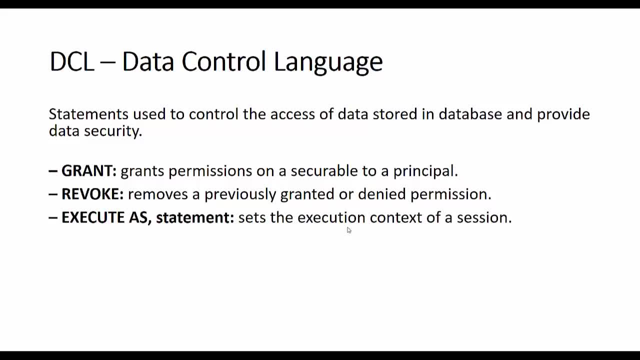 anything on that particular table. so with execute, as you can set the execution context of a session for a particular user, so you can execute a statement based upon some other user on on his particular user context. right execute as clause. so execute, as can also be used as a clause in the 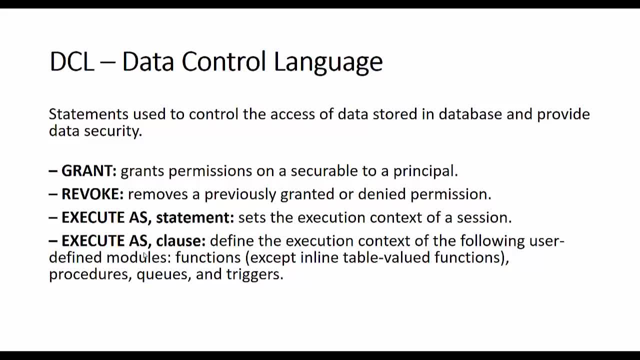 in the database object definition, like the functions and the stored procedures. so within the stored procedure you can use executors, execute as so. whichever username is passed on, that particular execute as so. the stored procedure or the functions will execute on behalf of that particular user by switching the context to for that particular user. okay, last one is the reward. 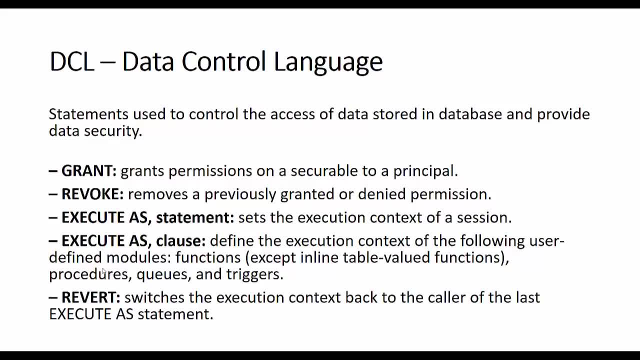 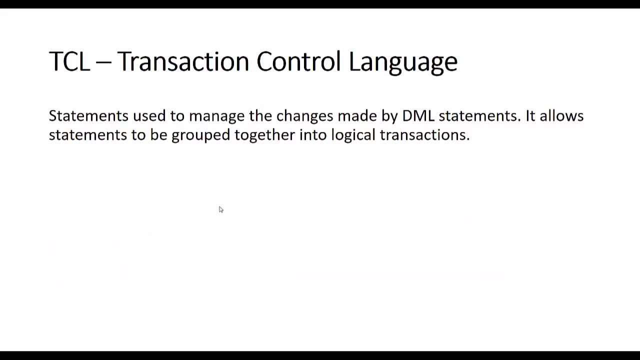 reward means whatever execute as context you have set for that particular user, it will revert to the original user that was logged into that particular session. okay, so reward basically switches back the execution context back to the caller of the last execute as statement. okay, the last thing is the tcl. 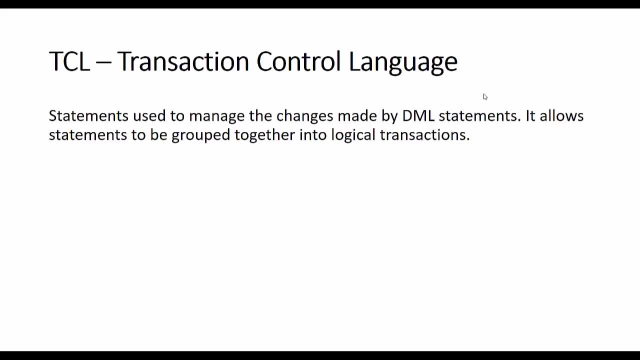 that is transaction control language. so transaction control language is basically the internal sql engine. how it basically behaves and how does it helps in maintaining the concurrency and the durability of the transactions. so this statement used to manage the changes made by dml statements. it allows statements to be grouped together into a logical transactions. okay, so. 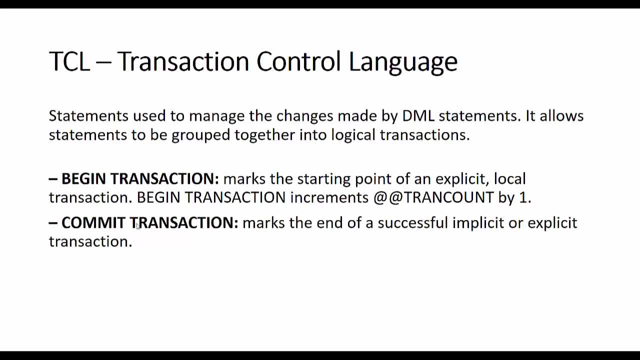 with the transaction control language. you have begin transaction and you have commit transaction and you have rollback transactions, so these three go together, okay, so when you are executing a particular statement so you can bind those particular statements within begin transaction and commit transactions. whatever statement is between those all, will you know, execute in a single. 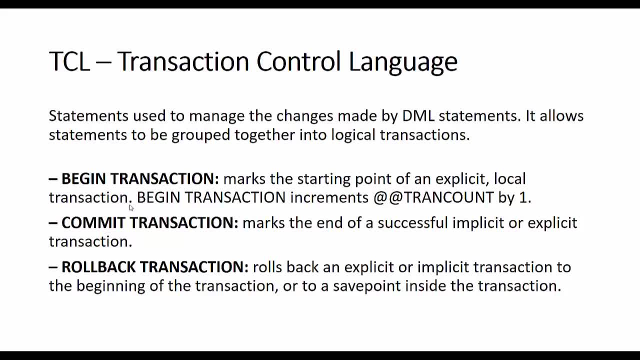 transaction. so either all of them will be executed or none of them will be executed. right, so begin transaction marks the starting point of an explicit local transaction. okay, so this transaction increments the tron count by one. the commit transaction marks the end of a successful implicit transactions. right, so complete, so commit transaction means that the transaction is committed. 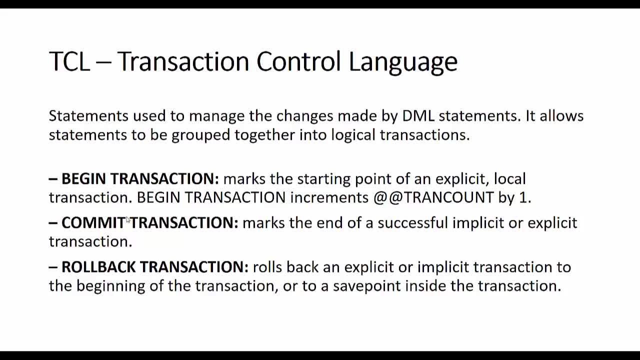 so let's say, within begin and commit transaction you have four insert statements, so they will insert four records at once and if anything fails in between, uh, they will roll back the previous uh insert statements that were done right, uh. third is the rollback transaction. it rollbacks the 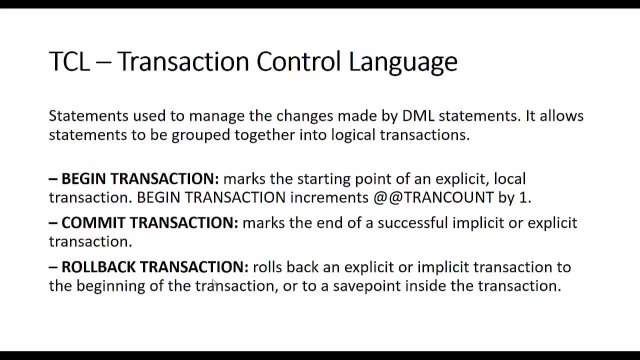 transaction that you have started right, begin transaction. it rollbacks the begin transaction if you have specified. and a third one is, and last one is the save transaction. so this tr, so this save transaction, creates a save point within a transaction, okay, so so all these things, uh, i'll. 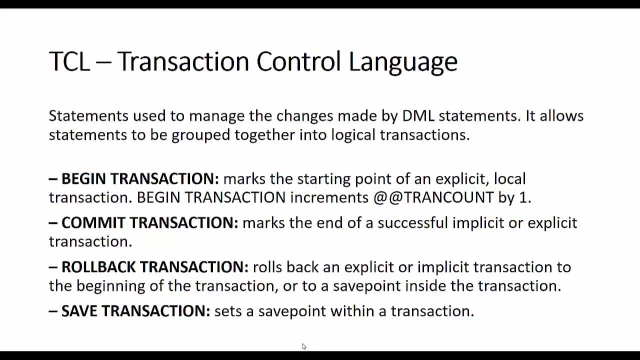 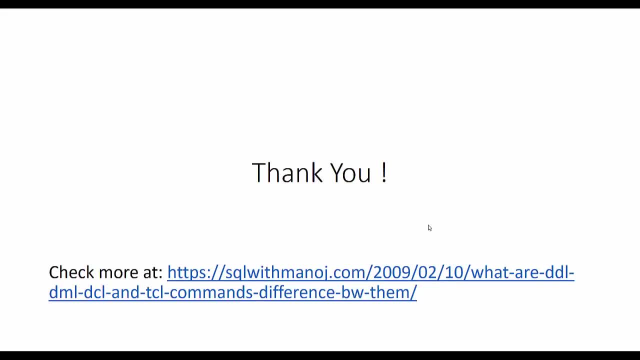 be talking in detail, but for this topic, this is just the high level overview i have given right. so i hope that you liked this video and please let me know if you want to know something in detail about these statements. so please subscribe this channel. whenever i add a new video, you'll get to. know about this. okay, thank you very much. have a nice day.